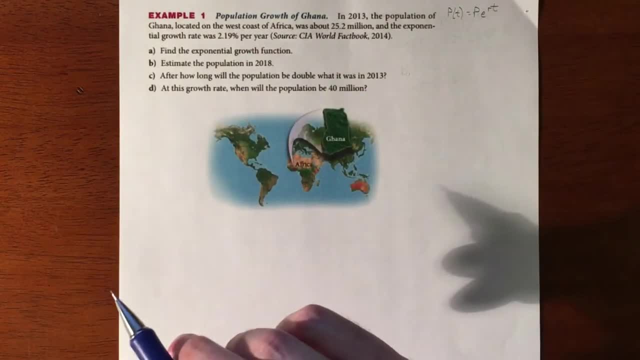 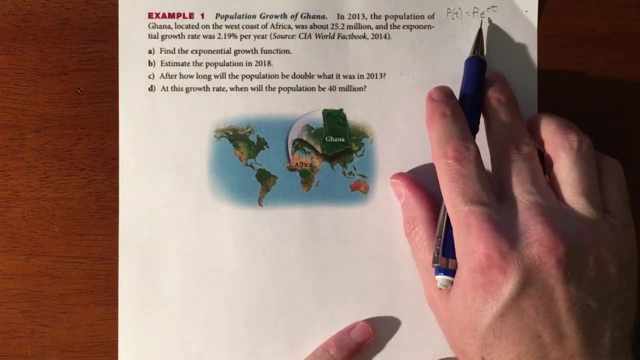 growing exponentially at 2.19 percent per year. So that means that we are talking about a population growth which changes continuously. So you're looking at a PERT type of an equation. So P represents our initial population, E is just. we are continuously growing, we're compounding. 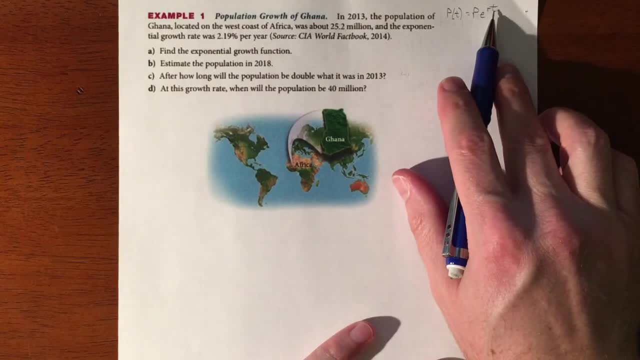 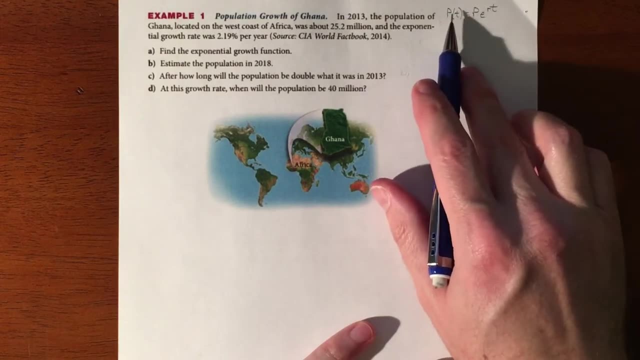 continuously and then rate we are given and then time is just some period of time. This represents your population after a certain period of time. So this equation is your population with respect to time. So as time changes it affects your population because your rate in theory is not. 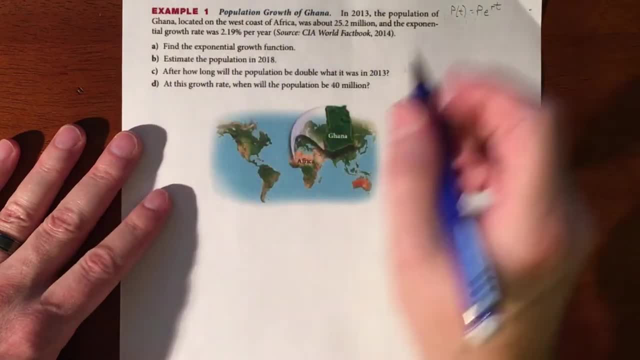 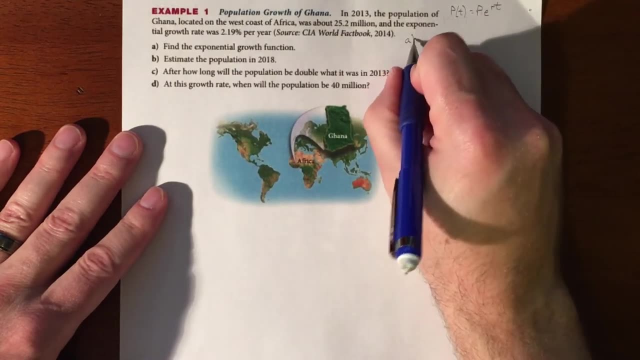 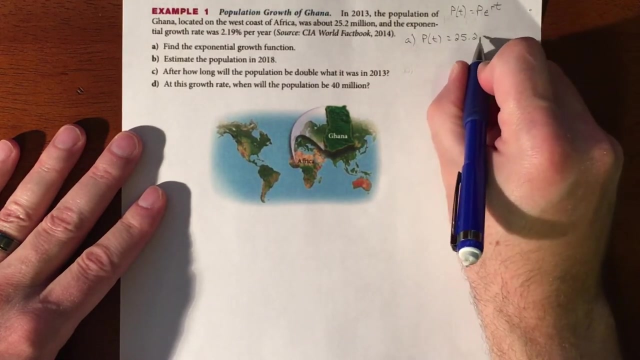 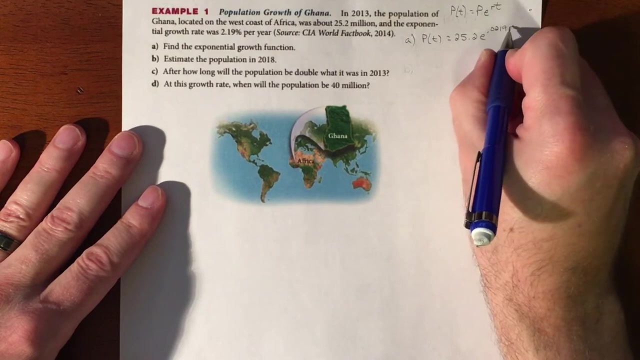 changing. So um, um. so what is the function? the exponential function for this equation We are looking at, our population with respect to time is going to be 25.2 million E, and then we want the decimal version of that rate, so 0 to 1, 9 t. Okay, so we're going to be. 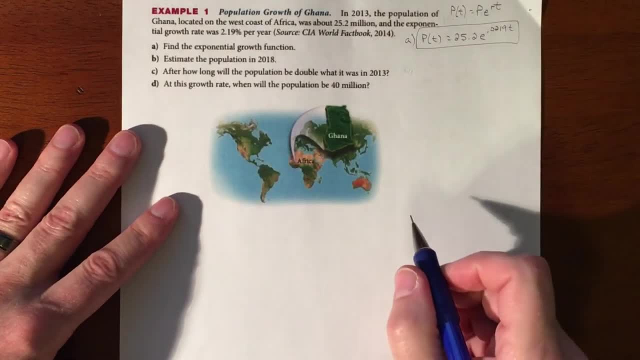 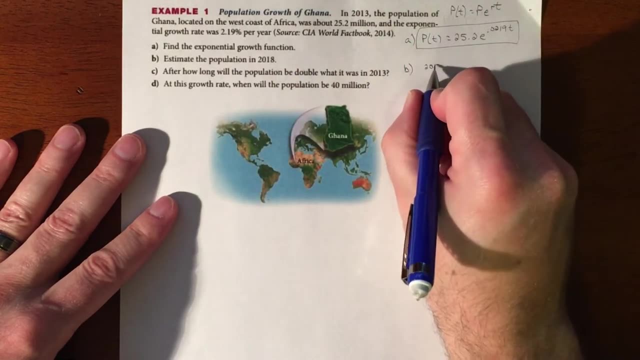 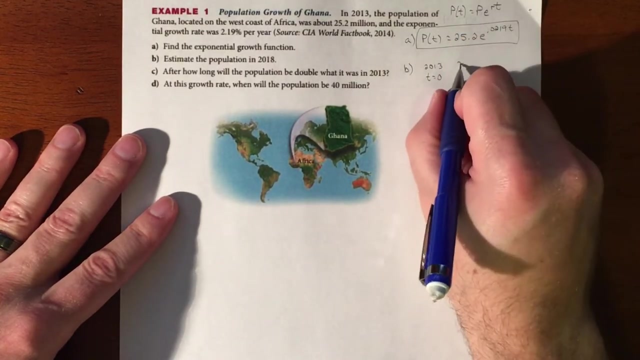 using this equation pretty much throughout all these different types of problems. So the second one is: they wanted to know what's the population in 2018? Well, if 2013 is our t equals 0, it's our initial population, what everything is based on, 2018 is going to be five years later. 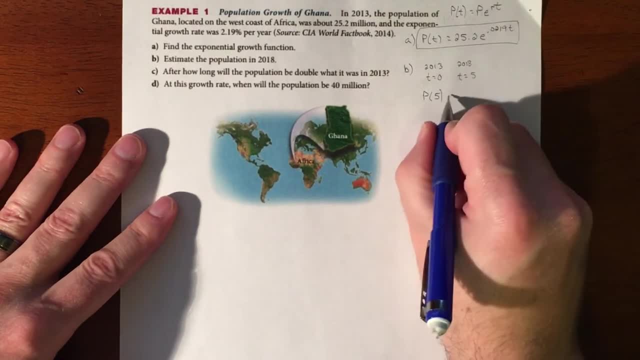 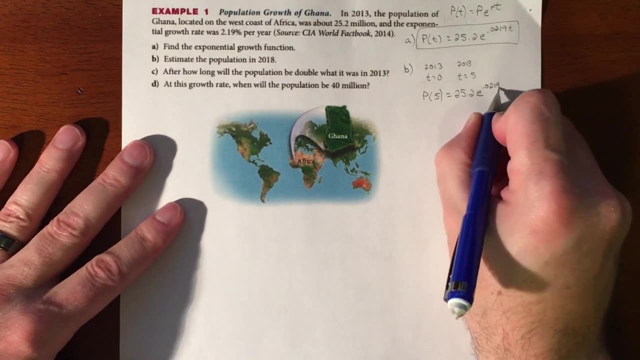 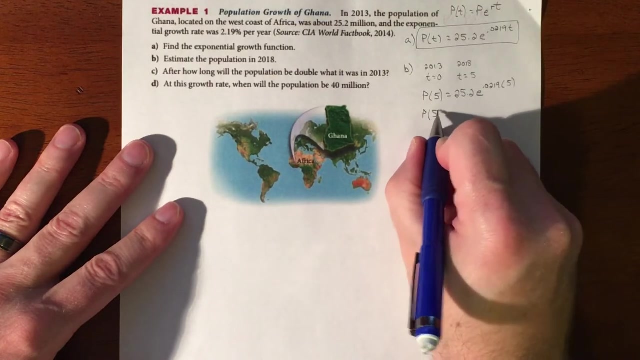 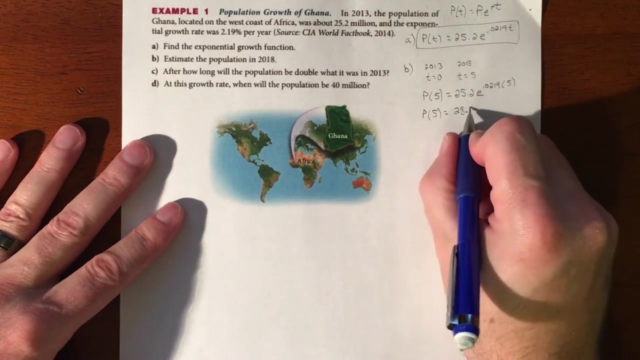 So we are going to do p of 5.. So 25.2 E to the point 0 to 1, 9 times 5.. So we are just going to plug that right into the calculator and our population five years after 2013 is going to be roughly 28.17 million. 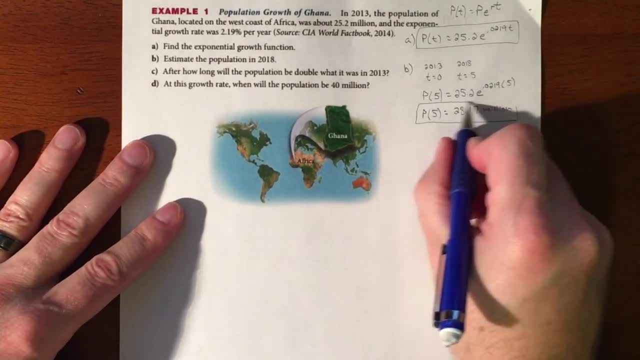 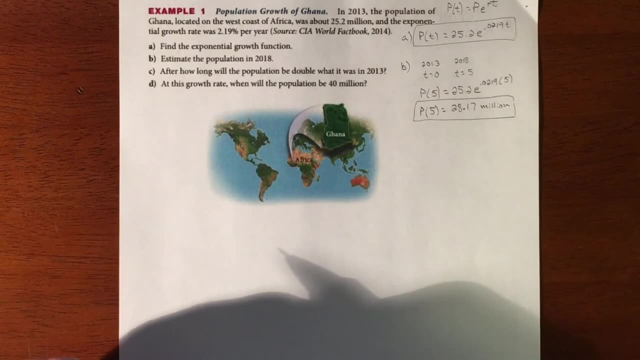 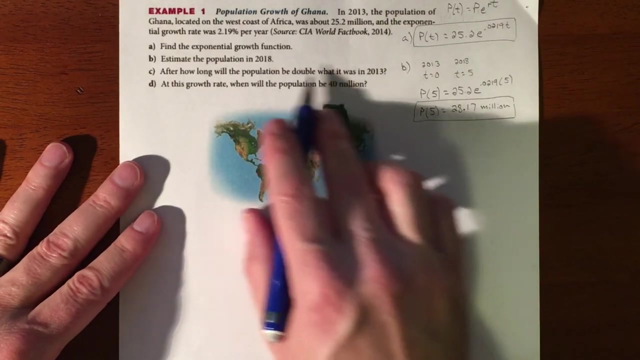 Alright. so next equation or next situation is: they are asking for: how long will it take for the population to double Um from 2013.. So, if it's growing at this rate, how long is it going to take to double? 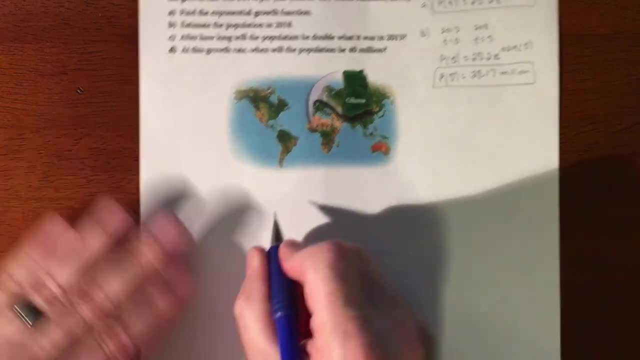 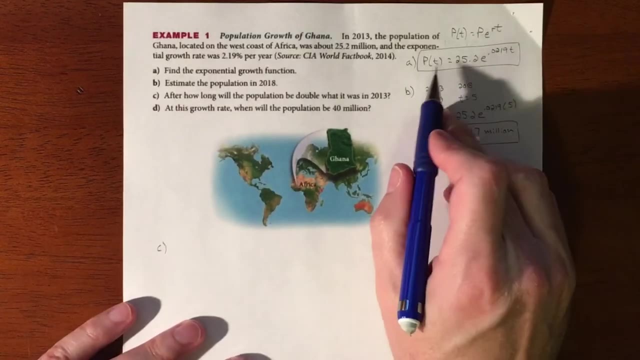 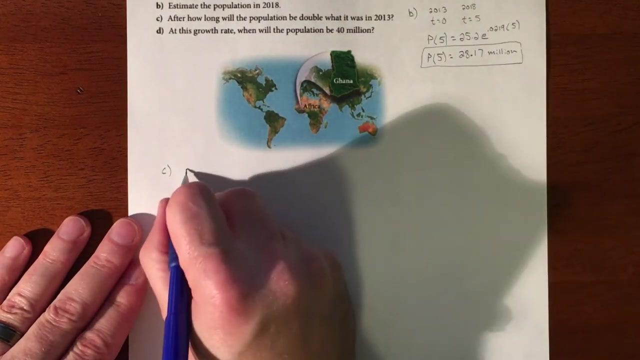 So if we do that, um down here, So we don't know, uh, the time, but what we do know is the double. So we are going to go from 25.2, our double is going to be 50.4. 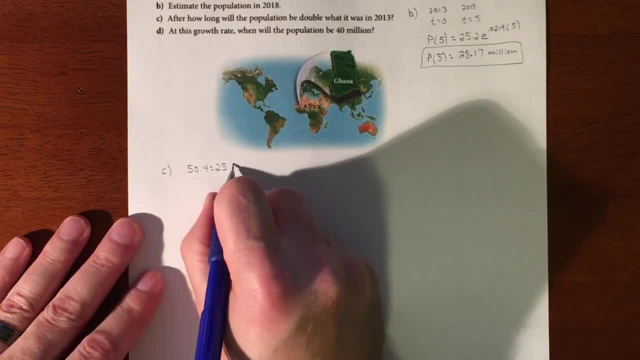 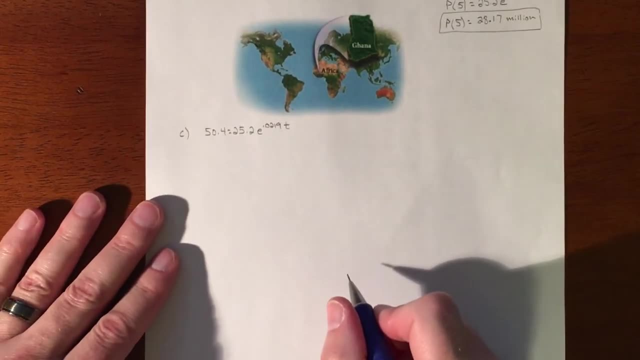 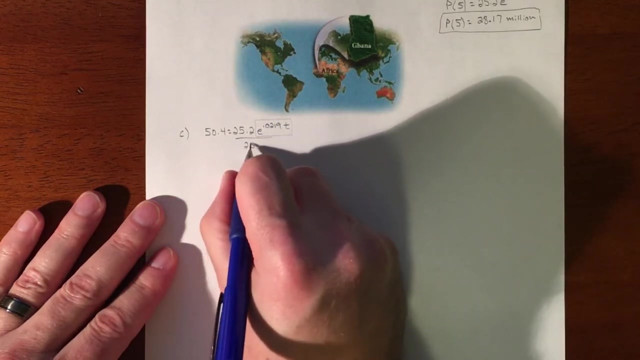 is going to equal our initial equation. But what we don't know is the time, So we are going to try to isolate this piece right here. So we are going to divide by 25.2, divide by 25.2, and that equals 2.. 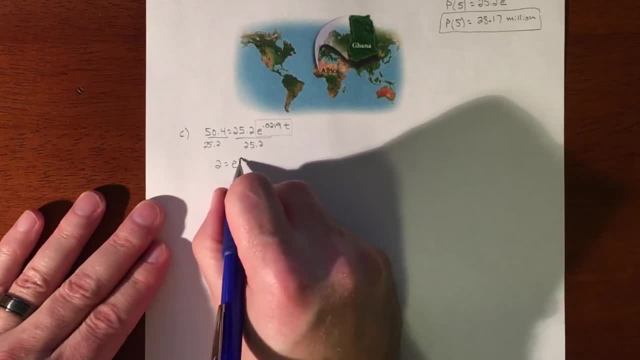 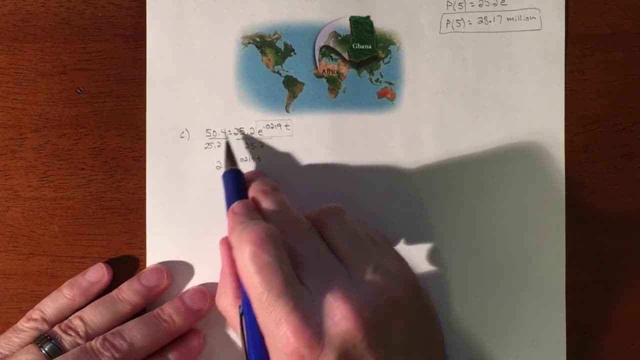 So, actually, if you are ever asked to double, triple, whatever the question relates to adjusting your population, if it's a really straightforward one, you can skip all of this, because every single time when you divide that over, especially if it's going to be a double, it's just going to equal 2.. 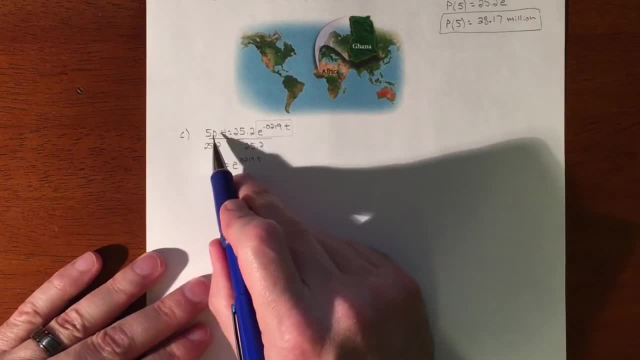 So it doesn't matter if you start with 1 and it's going to 2, you start with a million and it goes to 2 million. when you start to isolate this piece by itself, that's exactly what it's going to look like. 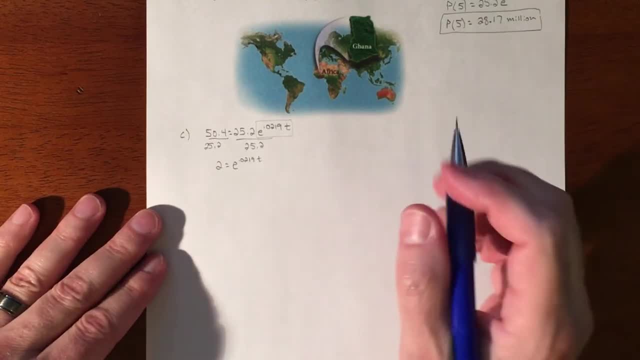 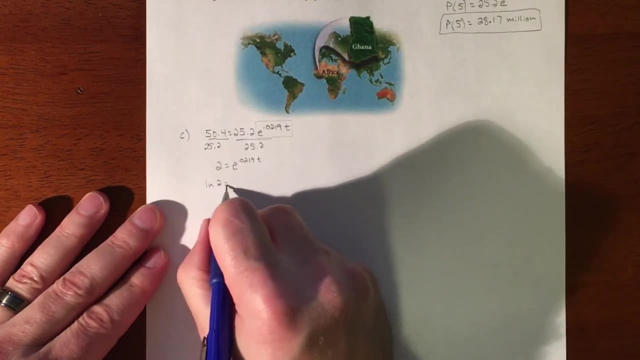 So you can kind of skip to that. If they're asking when it's going to triple, you can just do: 3 equals your equation. So, um, the way to solve this is we're going to log both sides And I'm going to natural log. 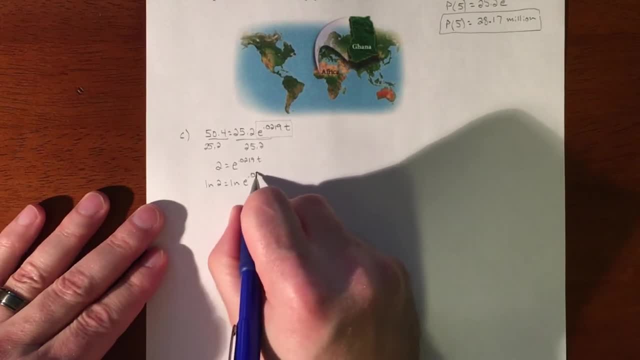 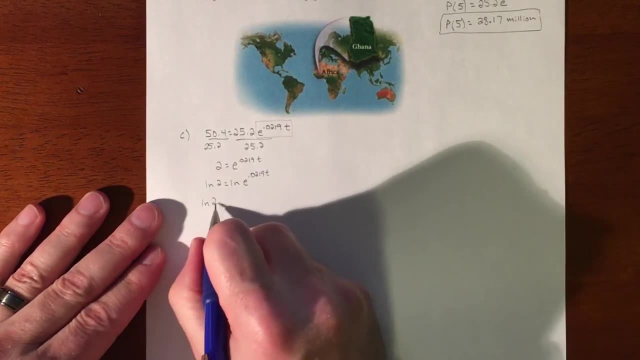 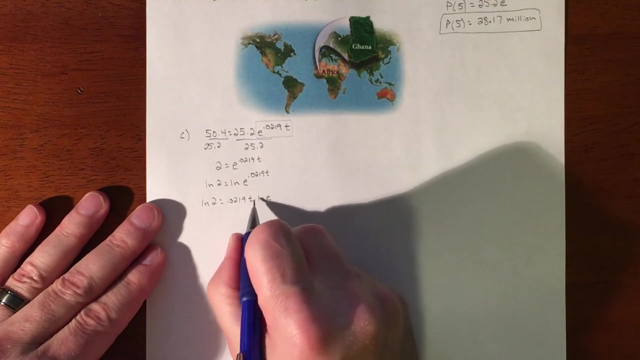 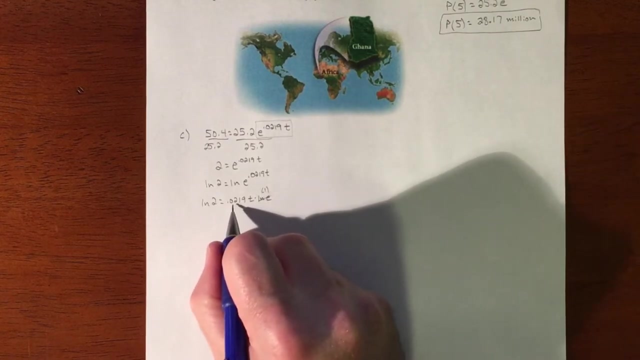 both sides, because this piece is going to work out pretty nice, And then the reason that we log is because this is going to come down Alright. so this piece right here, this natural log of e, is just 1.. So really, you're just left with this. 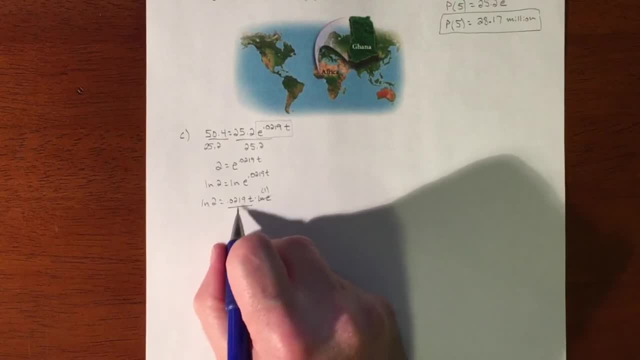 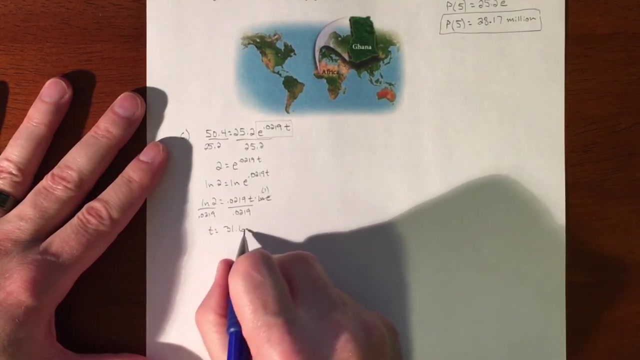 .0219 times t equals the natural log of 2.. So we'll divide this to isolate our t, And so we're getting t to equal roughly 31.65 years. So with the rate of growth of 2.19, um the population. in Ghana is going to be doubling roughly every 31 to 32 years if it maintains that same growth. Uh, last one, This growth rate. when will the population hit 40 million? So this is going to be um rather than us. 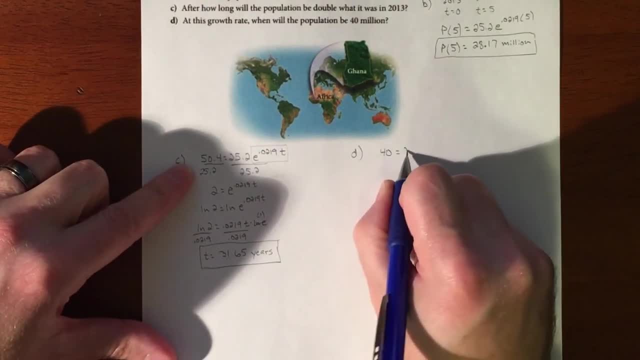 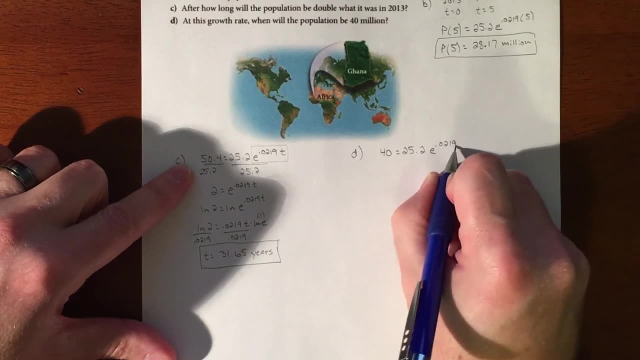 doubling anything. we are just setting it equal to 40. So this one's not going to divide clean, like I have no idea what's going to divide, But this is not going to be one where I can kind of shortcut that. So same kind of.